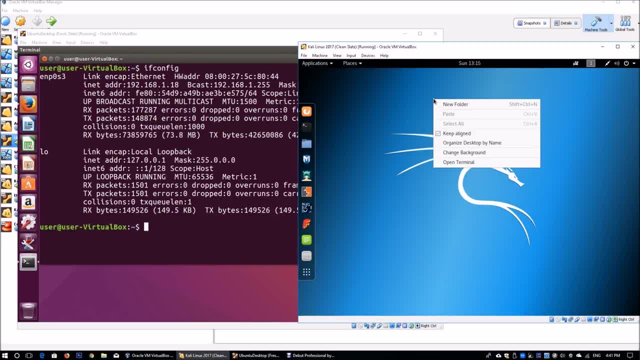 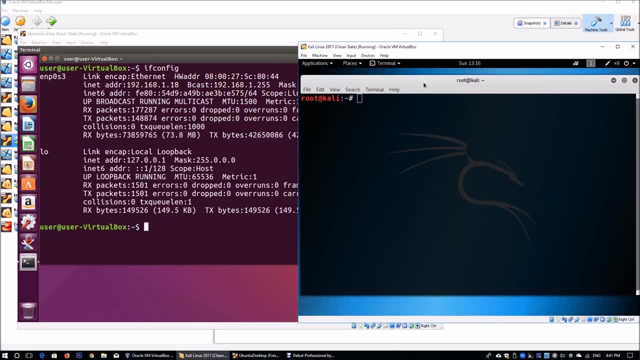 it's going to serve as the attacking machine. I'm going to close this over here. I'm going to launch a new terminal And in the new terminal I'm going to zoom in a little more So, again, it's easier for you to visualize what's happening. 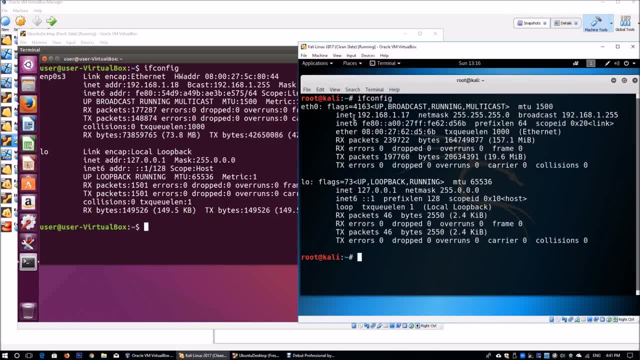 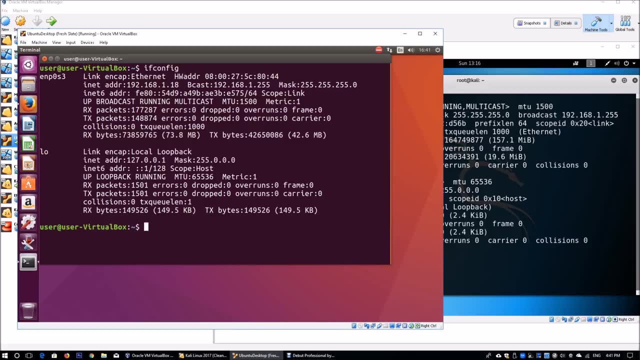 in the kind of attack we're attempting. So as I enter ifconfig, remember clearly we have an IP address from the attacking machine as 192.168.1.17.. So again, the tutorial for today is network intrusion detection system using Snort. So what we're going to do is we are going to go. 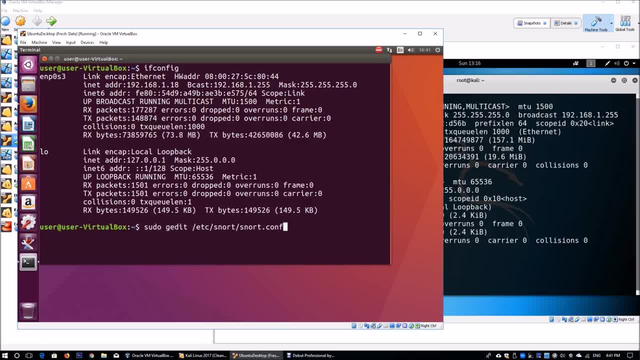 into ETC snort slash, snortconf. So this is the main configuration file of Snort. So we're going to validate, understand the configuration structure of the configuration file for Snort And then we're going to run Snort so that we are able to see the kind of detection that we can get. 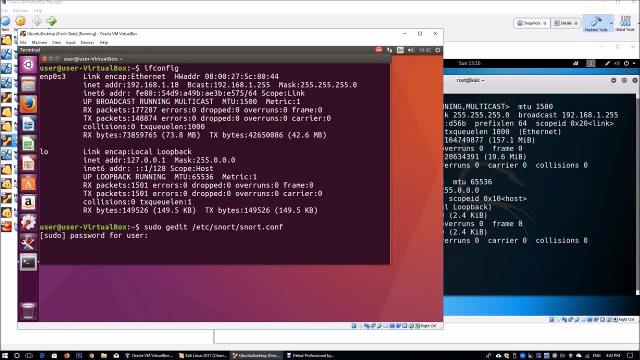 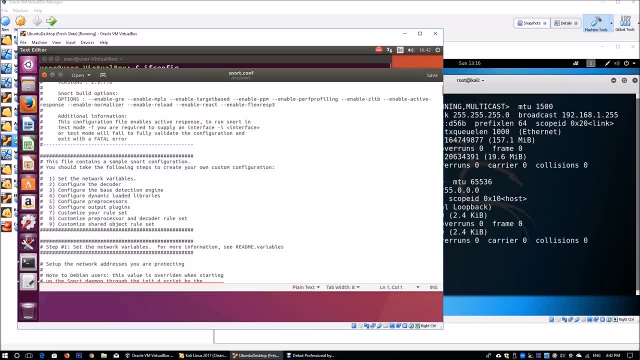 using the NIPS. So I hit enter. It asks for a password for my sudo. I enter the password for user And I go in. So over here we can see the file has a structure And in this structure there are nine specific segments. So you have network variables. You've got to configure a. 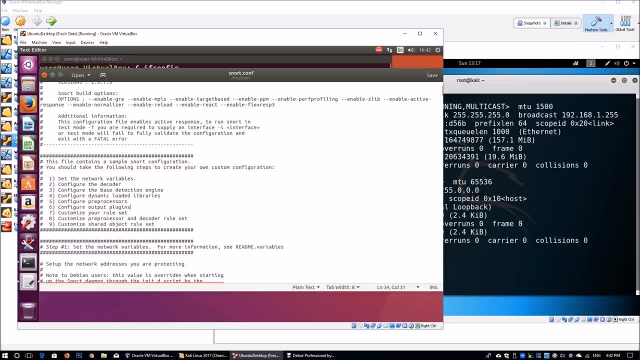 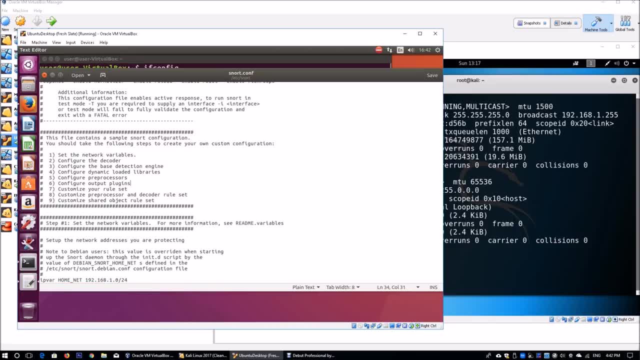 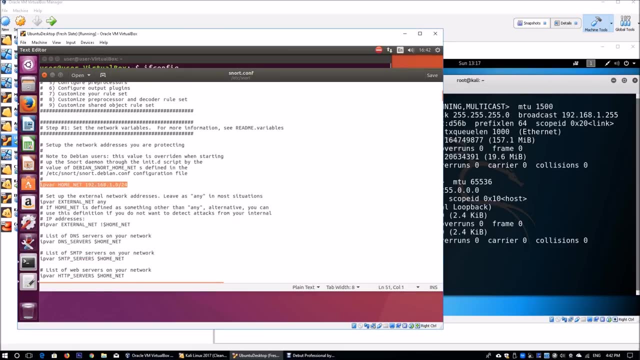 decoder, base detection engine and many other different capabilities for you to learn and to investigate on so that you are able to produce and maximize the value from the NIPS. So, as you scroll down, one setting that I have key in is home net is 192.168.1.0, slash 24.. So my home. 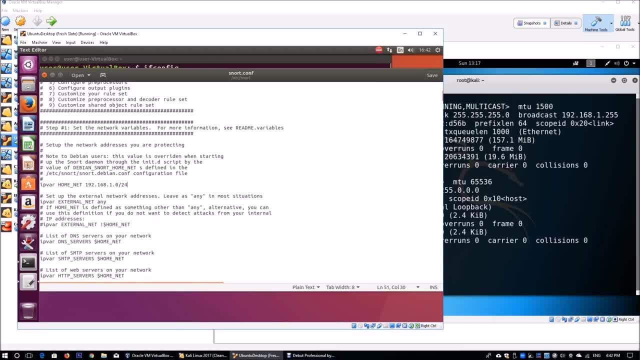 network on this testing lab environment is 192.168.1.0, slash 24.. So my home network on this testing lab environment is 192.168.1.0, slash 24.. So my home network on this testing lab environment that I'm running on is running on a variable from 1 all the way to 254 for the IP address of 192.168.1.. 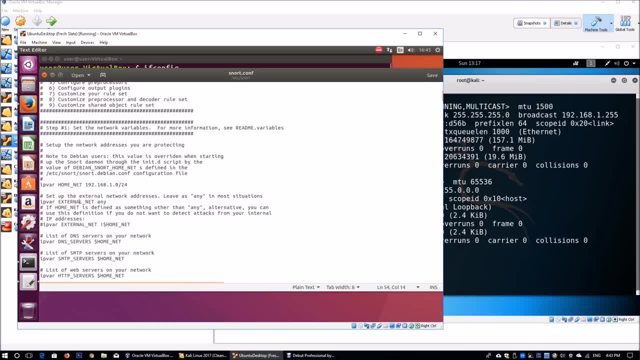 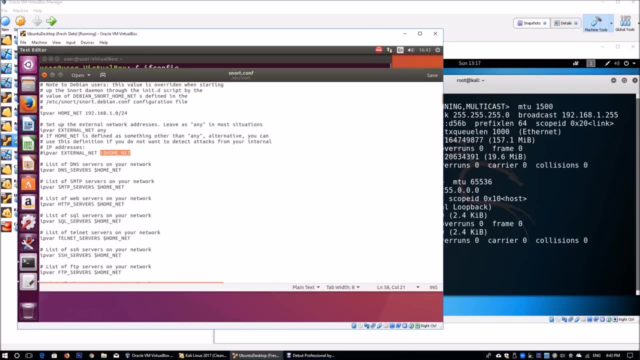 And, of course, external network. Again, if you're running on an enterprise environment, chances are your external network may just be anything outside of home. So in this case we have an example here that you can use. So this is the inverse of home network. And again, if you have DNS servers, 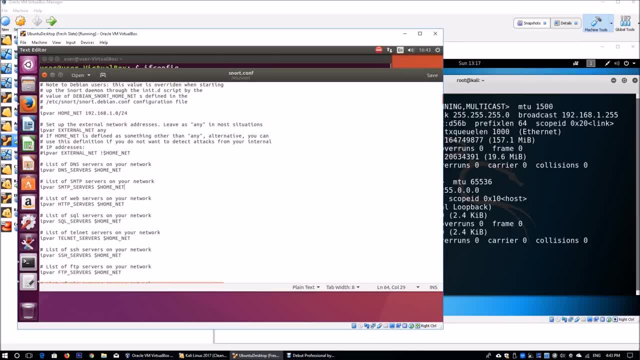 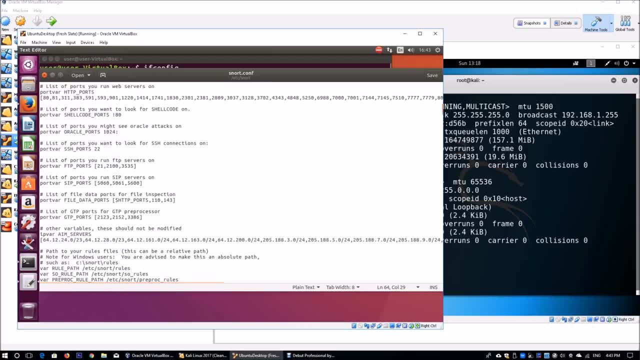 you can specify them. If you're an SMTP server, a 6TTP server and the likes. the configuration can grow more complex as you get larger. But one important case I want to really take note of are the rules. So over here we have a rule path that we have set as a variable. 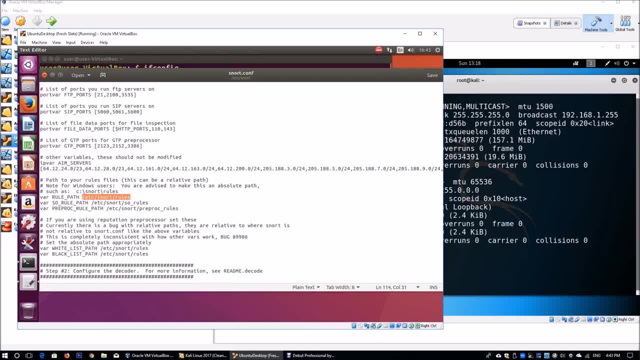 and it's in the folder of etcsnotcom- slash rules. So this is an area where we're going to explore a little more on, because it's critical for the rule setting, the policy setting, so that the security policy that you place in it allows you to detect a different kind of attacks coming. 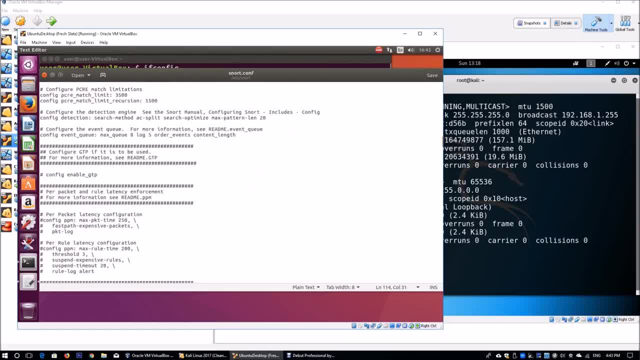 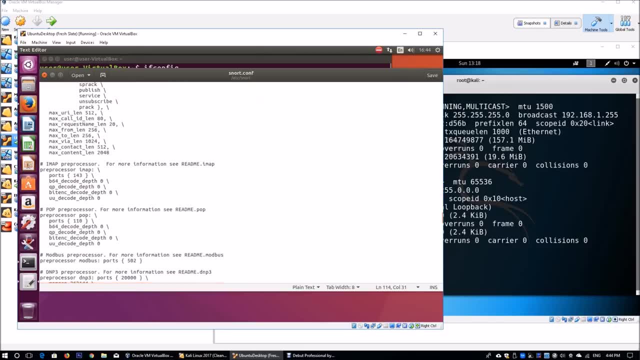 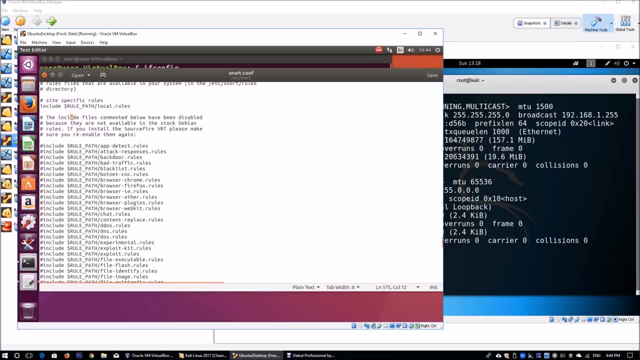 in So as we scroll down, what's really important is the list of rules that are available for you to actually use, the lies that are available from the community that are available as smart of snort And over here, for example, we can see the kind of different files that you can input in. 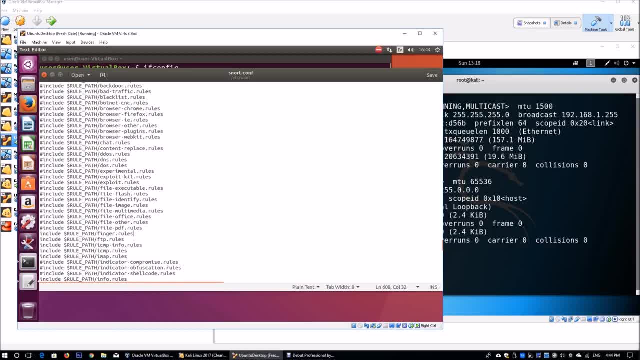 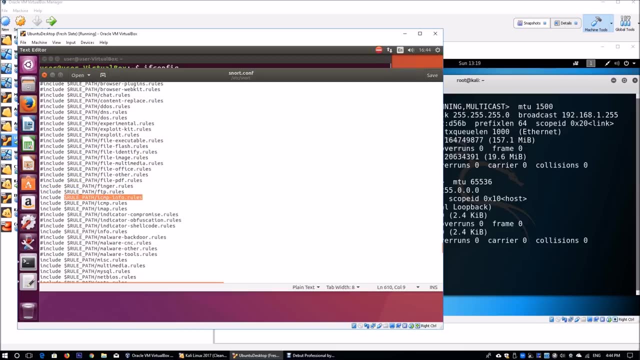 and you'll be able to activate them and they will be able to find out information whenever you want. So over here we got DDoS, we got DNS, but they are all commented out. So what is being in part of the rule engine is actually the fingerrules: FTP, ICMP, IMAPS and the like. 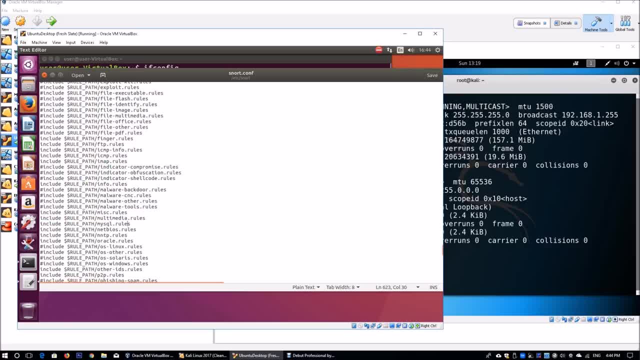 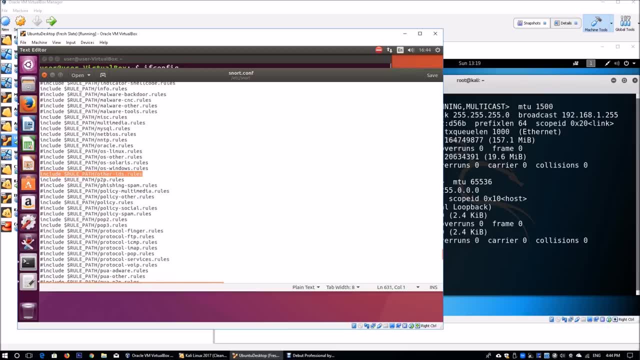 information, some miscellaneous Multimedia, MySQL, if you're running SQL, if you're running Oracle databases, you're running Oracle Solaris. Again, you want to enable all these policies that are relevant to the system that you're monitoring. And again, if we go in depth into 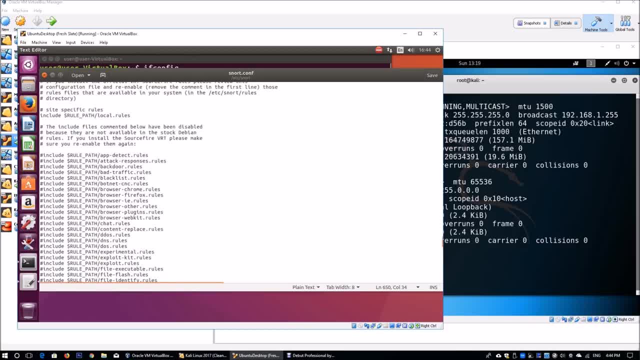 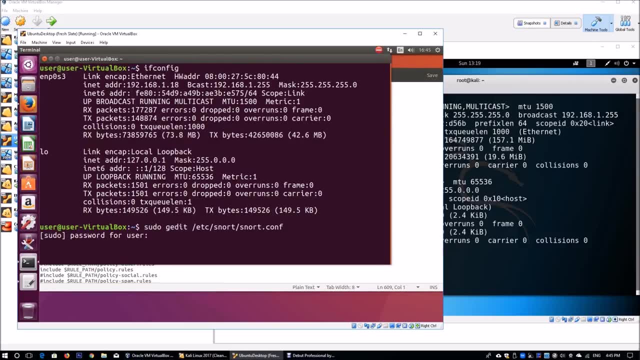 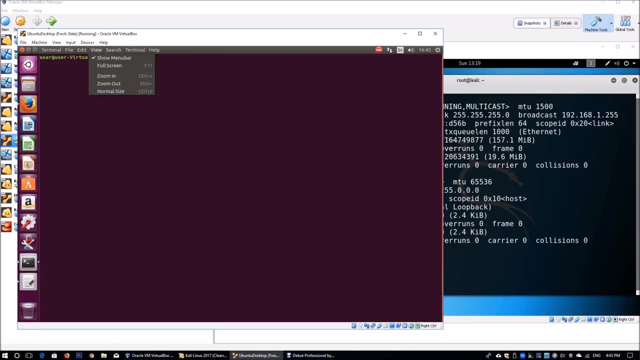 for example, some of the rules here we'll be able to see what a kind of traffic policy that they input in. So, for example, if I were to go into this path over here, so I'm going to open a new terminal Again, I'm going to zoom in a little more Over here. I'm going to click onto the view. 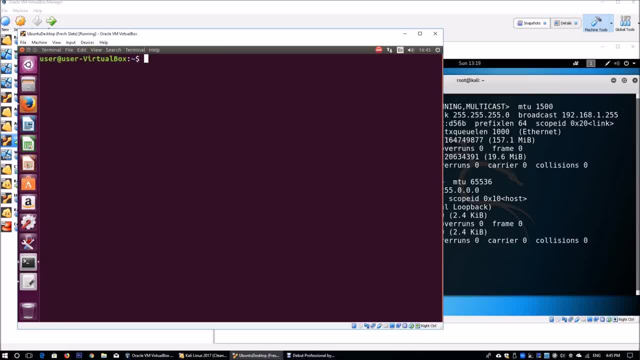 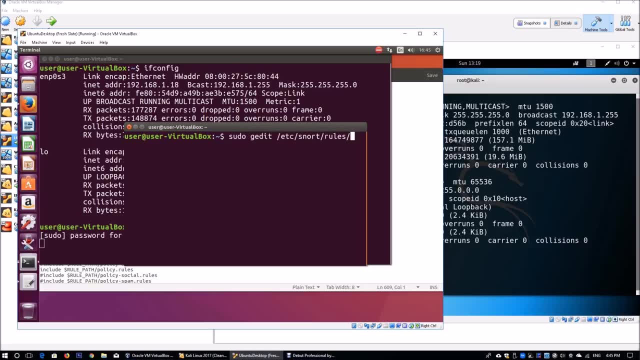 zoom in and zoom in a little more, And over here, what I'm going to do is I'm going to do a sudo, gedit, slash, etc. snort, slash rules, slash, for example, the FTPrules. So when I enter, and of course I enter my password to access the file, 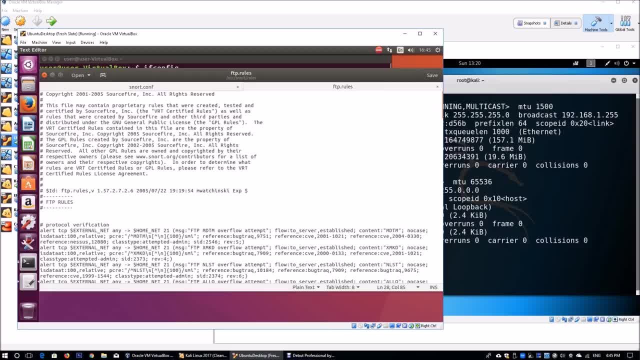 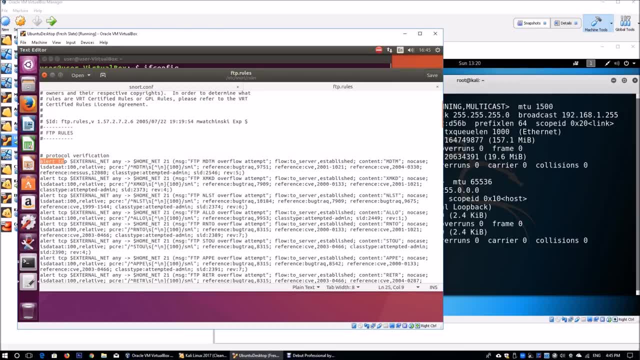 So once I go in I see a new file that's opened up And over here you have all the rules that are available as part of the verification. So in this case we have alert of a TCP coming from any network, from any source destination, And then from here we can see the port number 21 coming. 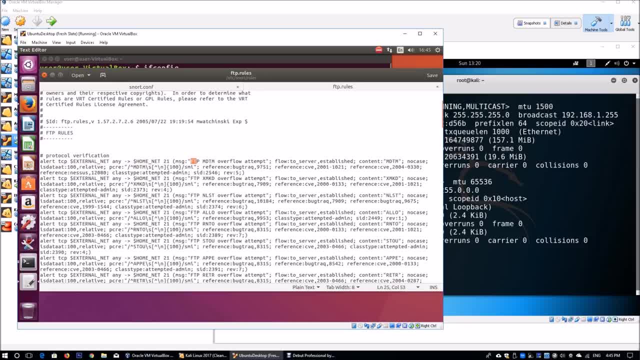 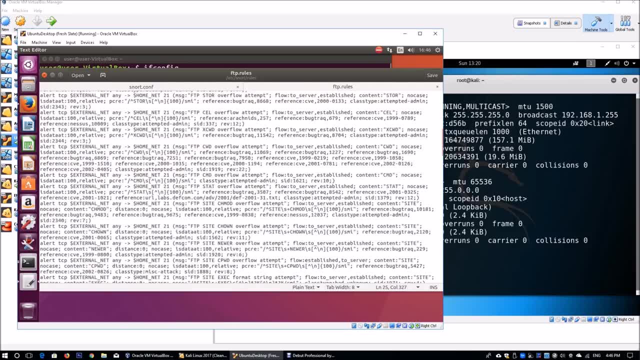 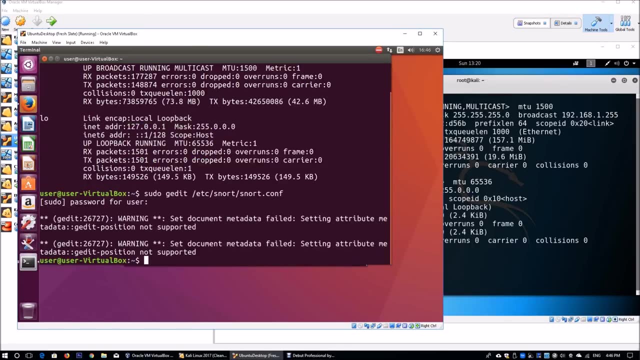 in, We can flag them out, We can put a message that is: FTP, MNTP, overflow attempt, and the like. So again, we are trying to find out the different kind of attacks coming in so that with all these rules, all these signatures, we're able to detect the cyber threat. So, as I continue into the 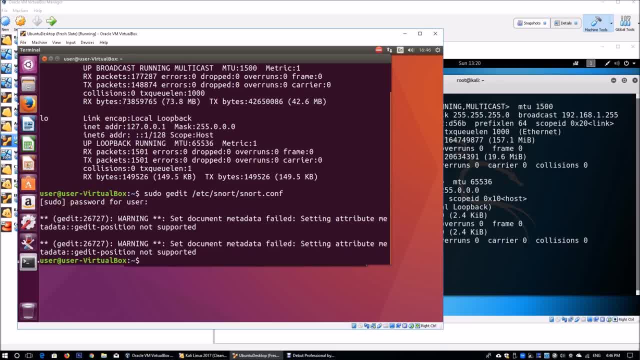 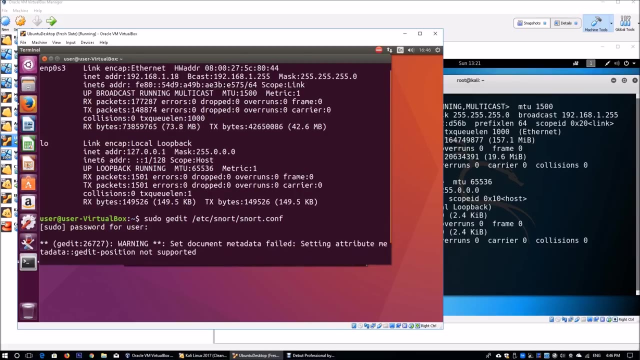 demonstration of technology. it's very important for you to understand how many of these rules work. So what we're going to do now is we are going to do a testing. So I'm going to do sudo snort, dash, ks, capital T, dash c, etc. snort, slash, snort, dot, configuration, dash i, emp0s3.. So emp0s3 is the. 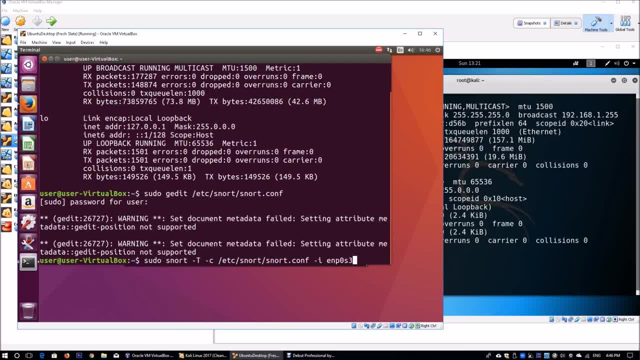 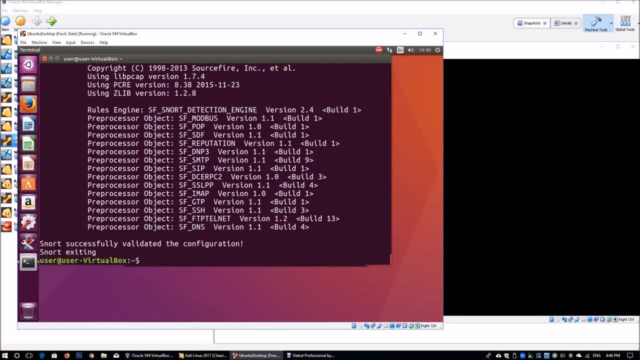 network interface card that I'm running on. So again, if it's yours, chances are it's going to be different. So when I do this, it will allow me to test whether my configurations are proper. So only when my configurations are proper will I be able to run snort. If not, you've got to. 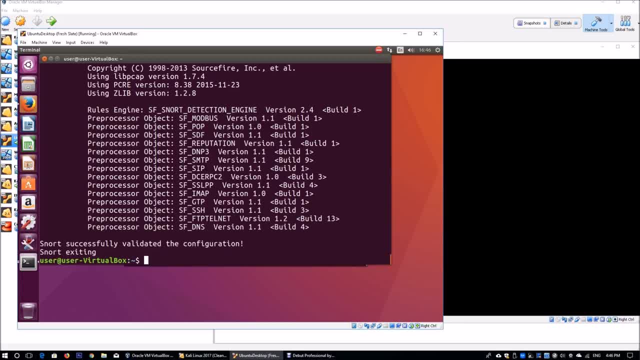 validate the configuration, Make sure that the parameters you're putting in are correct and proper. So once we have tested the configuration and it's good to go, all you got to do is enter sudo: snort dash a console dash q dash u snort dash. 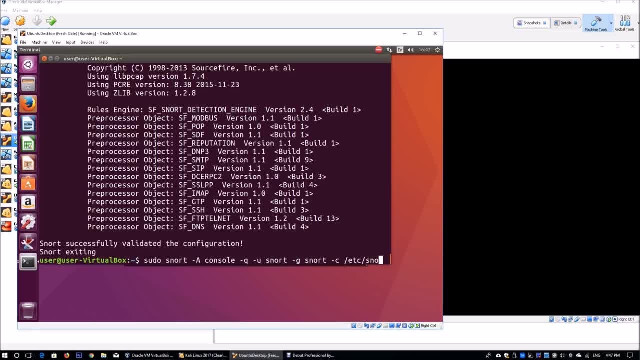 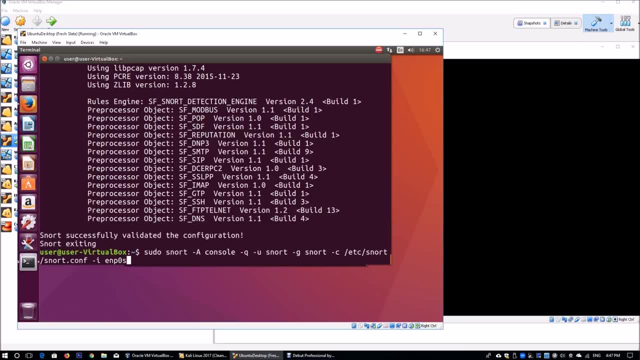 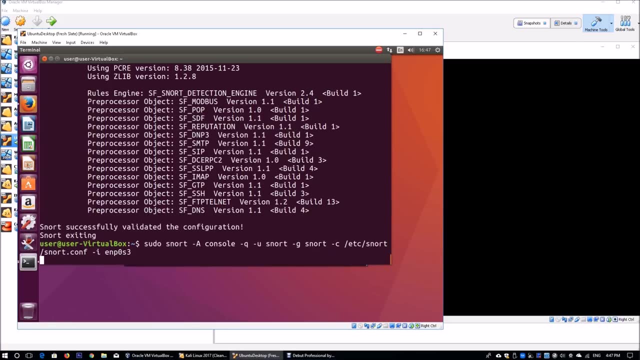 g, snort, dash, c, etc, snort, and then pointing to the configuration file again, And then, of course, your interface card that you are monitoring, And from there you will be able to start monitoring, which is the cyber attacks. So I'm going to go back to my Kalo Linux now, now that I've enabled 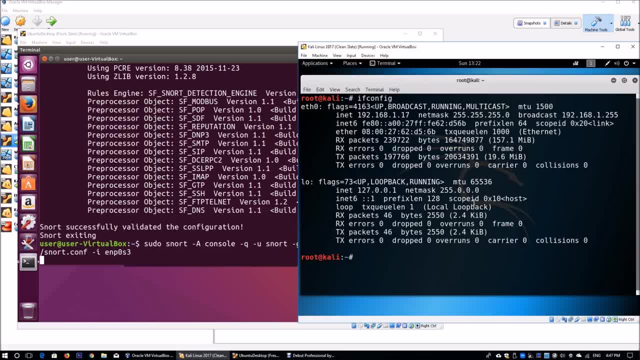 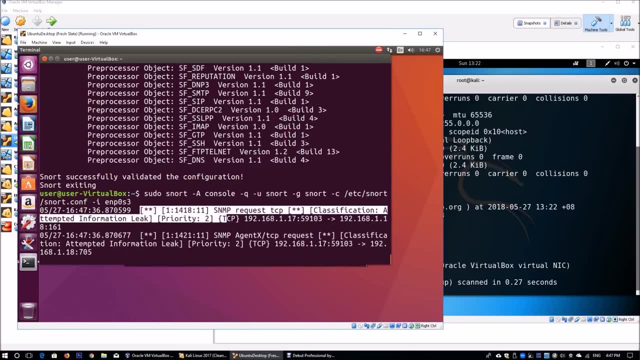 the monitoring on the Ubuntu operating system. So I'm going to do, for example, a direct network mapper scanning onto 192.168.1.18.. And what's going to happen is it's going to pick up directly the kind of attacks that's coming in. So over here we can see SNMP requests: classification. 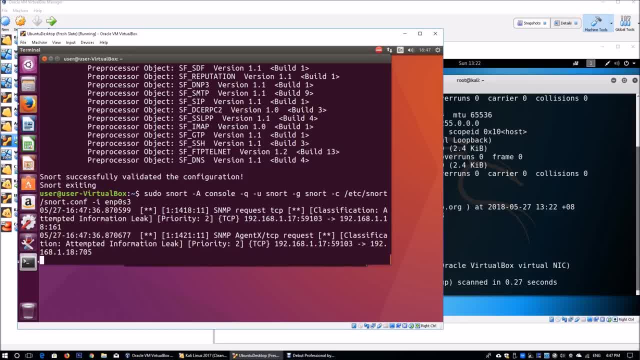 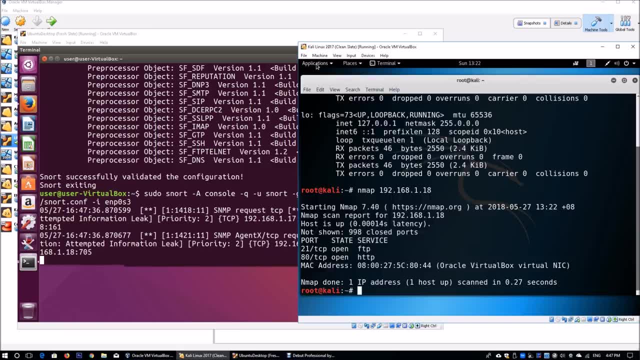 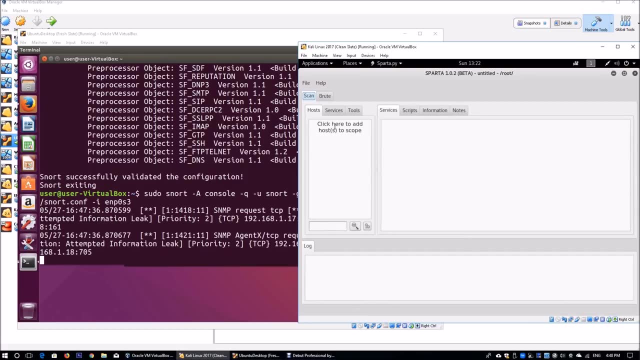 is that this is attempted information leak And again we see another attempted information leak against the operating system. So if I was to turn on another information gathering tool, like, for example, if I turn on Sparta, so Sparta is a great GUI tool that runs all the different. 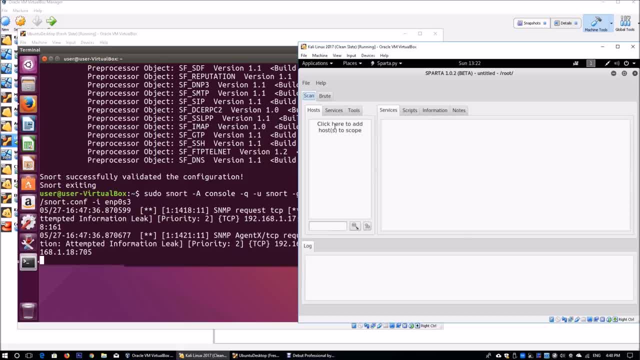 kinds of reconnaissance attack on Kalo Linux against the operating system. So I say I want to target a specific IP address, which is 192.168.1.18.. And I click Add to scope. And once I've added the scope, 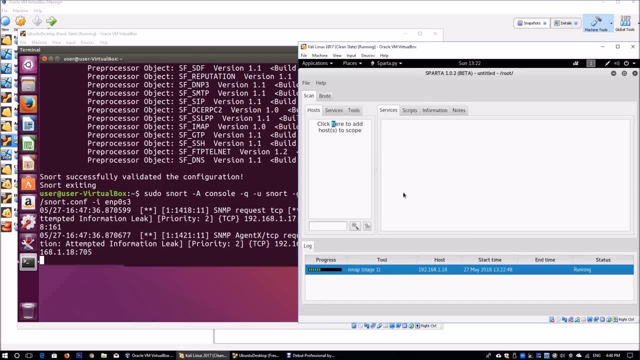 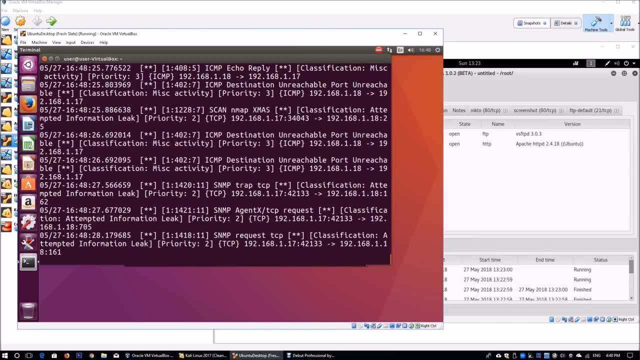 all the scanning on Nmap. you see it's on stage one, it's running multiple services, it's beginning to kickstart different services And we see that on the backdrop, we see that Ubuntu is detecting all these different kinds of attacks coming in And of. 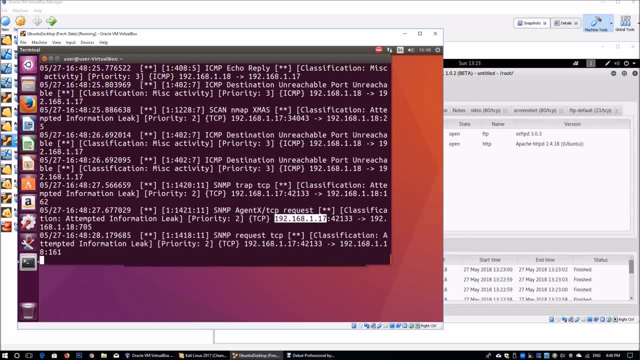 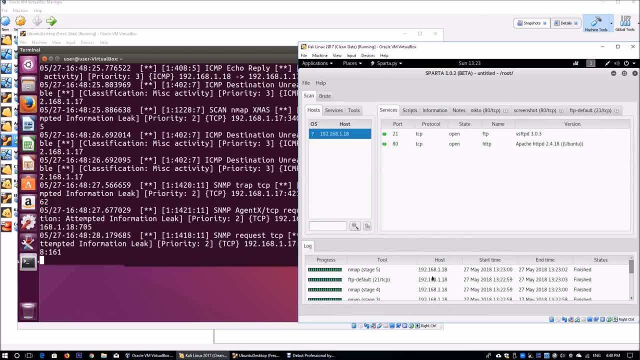 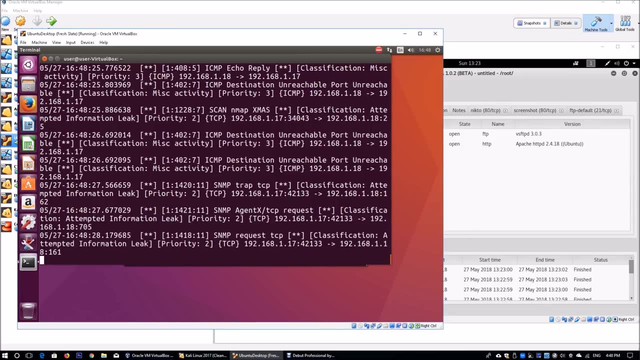 course we see the IP address of 192.168.1.17,, which is the attacking machine against the destination of 192.168.1.18.. So we are able to perform the scanning attack against the operating system And then, of course, we are able to detect them And we're able to respond to this type of 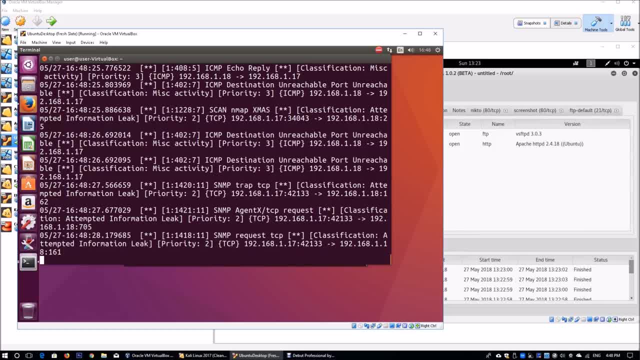 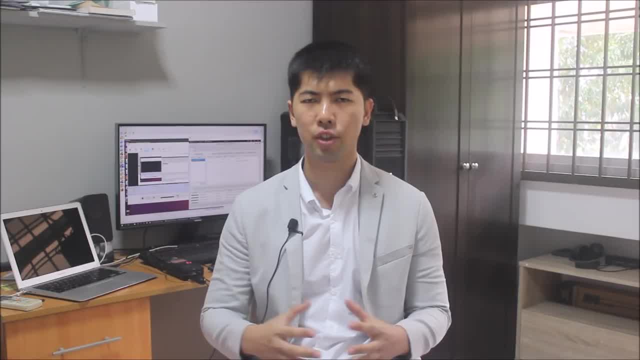 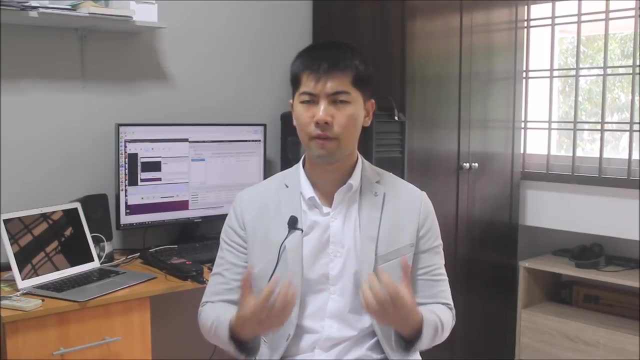 attacks, either by disabling the service or by stopping the attack altogether in a network. There you're seeing, we have used a software based network intrusion prevention system and we're able to detect a different kind of scanning, reconnaissance in the environment And, of course, if you were to try to use buffer overflow attacks, if you're trying to do SQL. 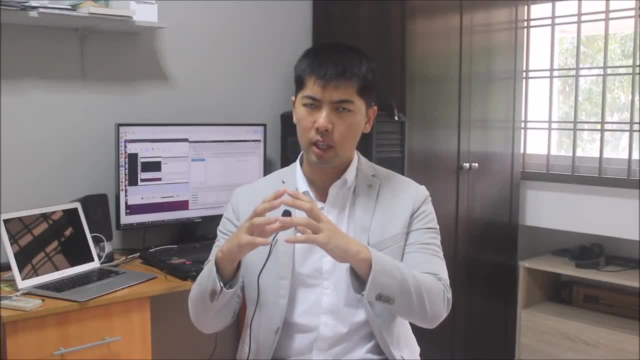 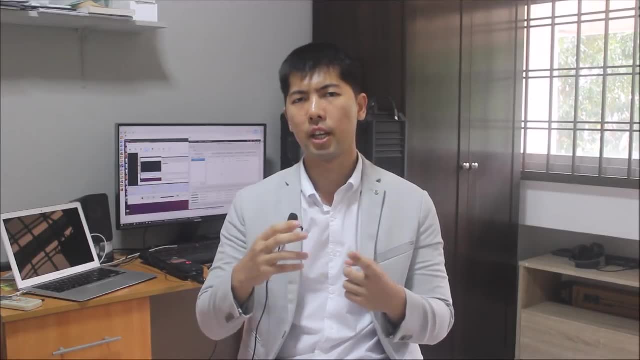 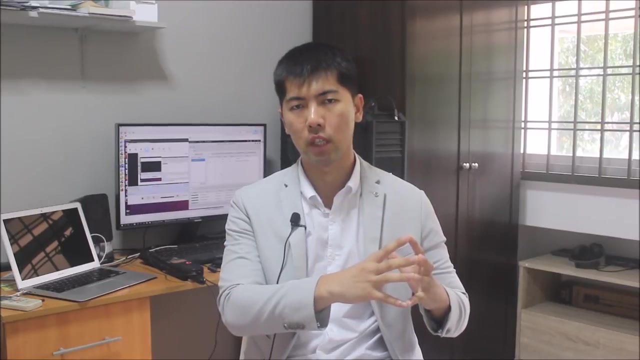 injection. there are rules and policies that are specific and designed for certain application servers. So one of the rules that you can see under the configuration file is actually a server Apache. So we are specifically designing rules and policies to actually protect a kind of web application server And from there the different rules will be applicable to this. 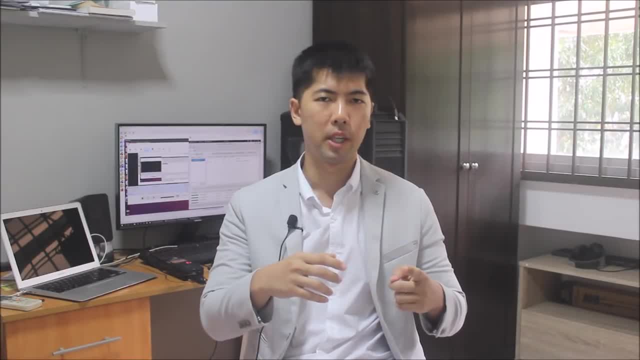 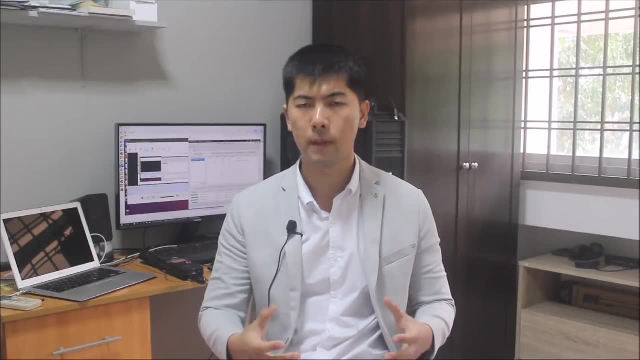 application server so that you can properly defend against it. So it could be a certain kind of file traversal, it could be a certain kind of injection coming in a cross-site scripting request, cross-site request forgery. Again, we're able to pick it up within the operating system. 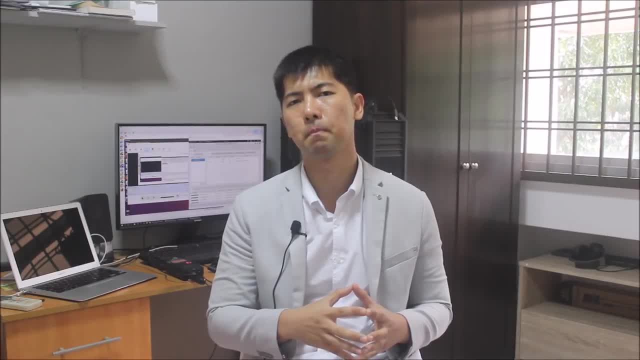 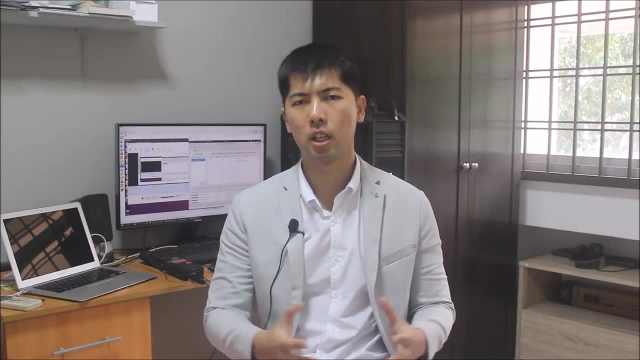 through the use of SNORT as a network intrusion detection system And, of course, in large-scale enterprises that you are deploying on. you have many different servers. Your servers could be residing on the DMZ zone. Your servers could be residing on the sub networks. So again,